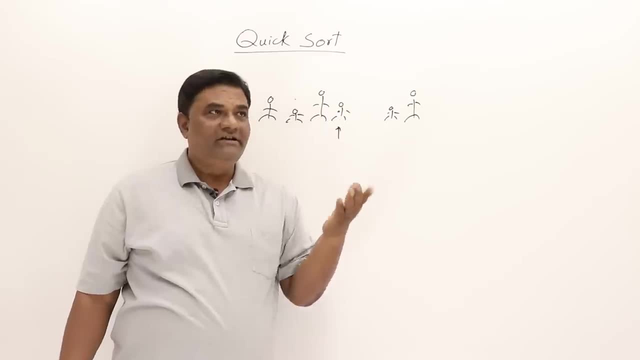 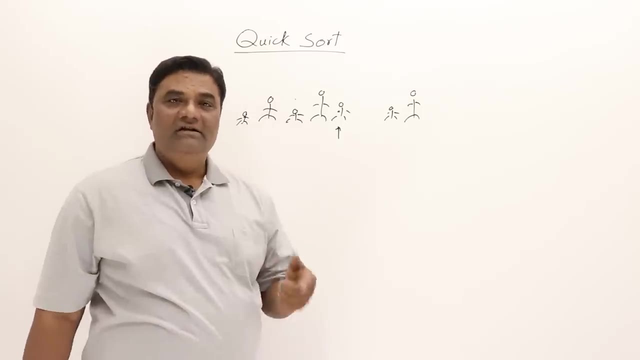 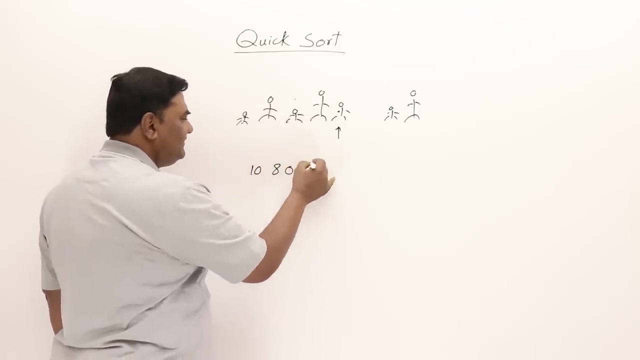 I will see that the person who is taller, he should be at the back of me, So let him go at the back and shorter person should come in front and I will find my place. That is the idea of quicksort. Now I will write few numbers: 10, 80,, 90,, 60,, 30, 20.. Which element is the most important? 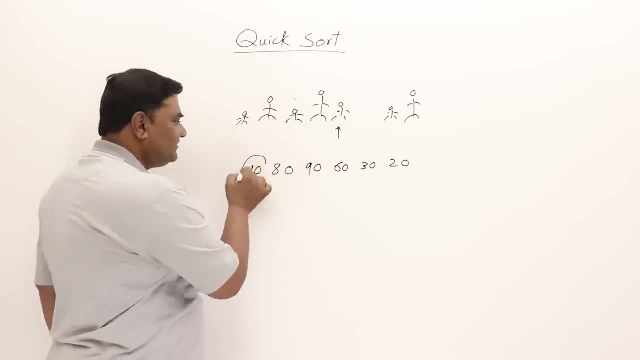 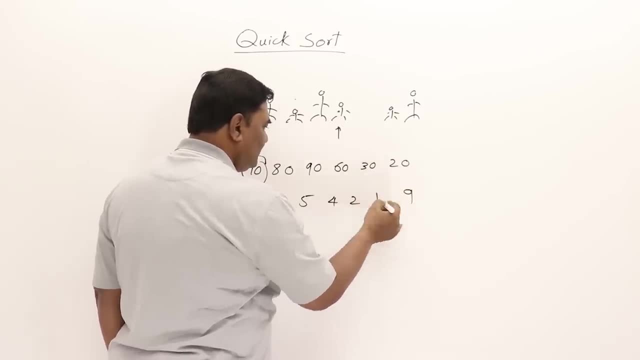 9. Which element seems to be sorted in one glance, if you see Which element is the most important, Which element is the most important, Which element seems to be sorted in one glance. if you see This element is sorted, How we can say that. 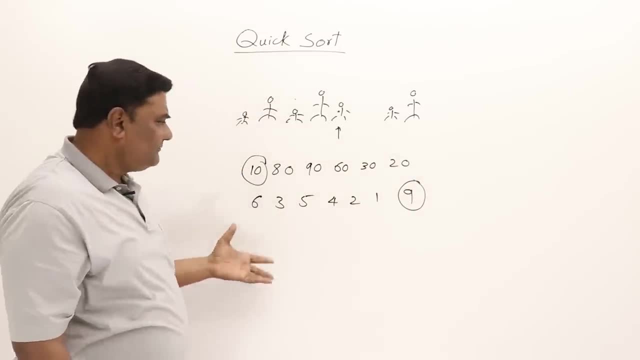 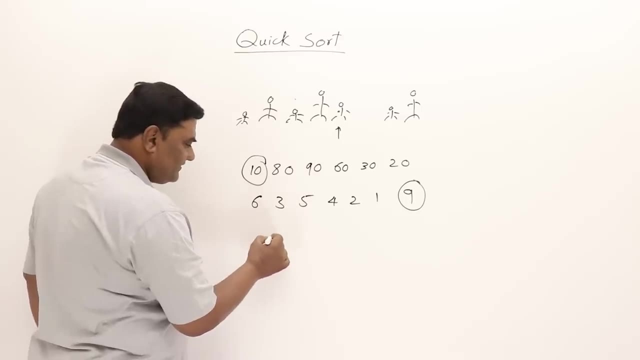 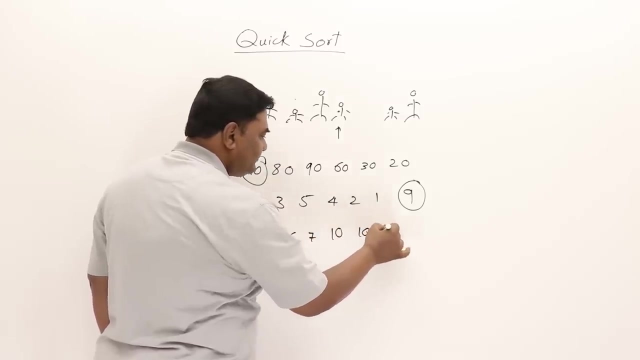 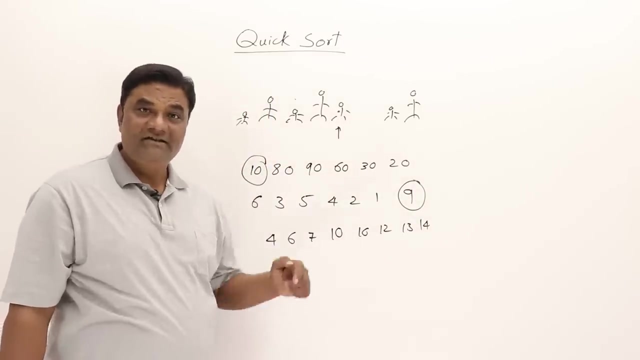 That is largest and it is at the back. Rest of the numbers Don't know whether they are sorted or not, but that is sorted In the same way. if I have the numbers 4, 6,, 7,, 10,, 16,, 12,, 13,, 14, which element seems to be sorted in its sorted position? 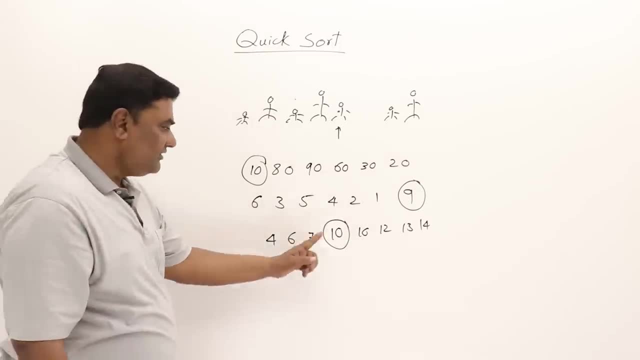 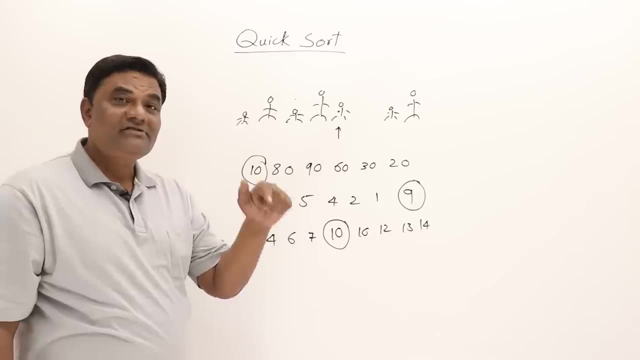 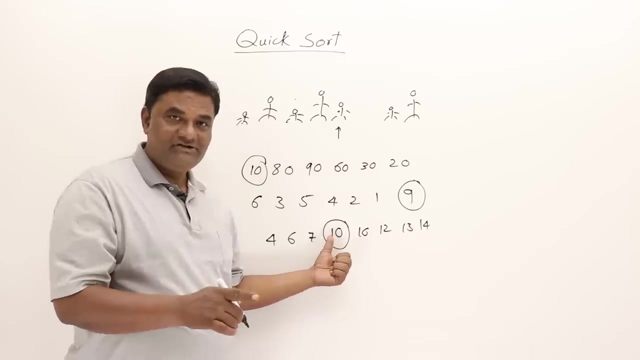 this element is in sorted position because all the elements before that element are smaller than this one and all the elements after that element are greater than that element. so that is it sorted position. so quickSort works on the idea that an element is in the sorted position if all the elements on the left-hand side should be smaller than that element all. 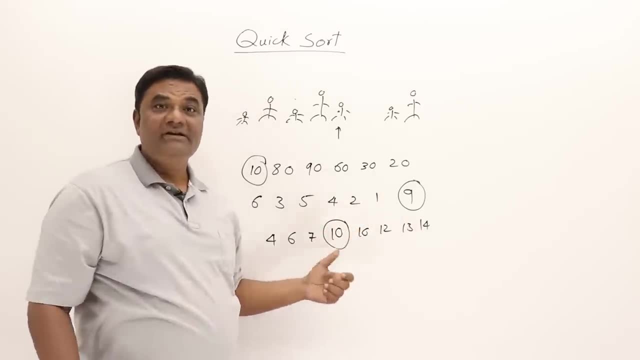 the elements after that element that is on the right-hand side should be greater than that element, then that element is in sorted position. rest of the elements may or may not be sorted. so this is the idea of quickSort. quickSort works on this one and that is how. 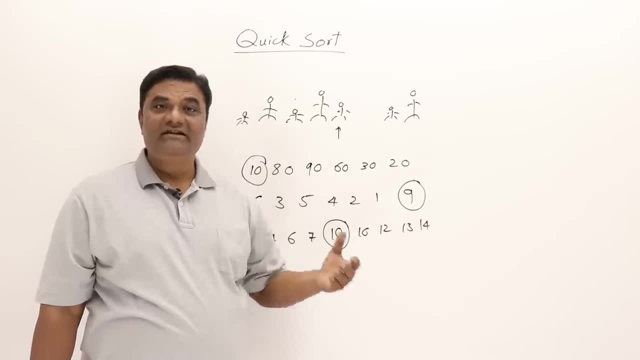 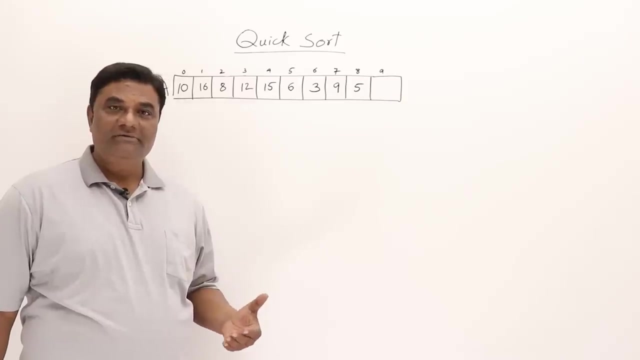 the name comes quick, so, like a, students can quickly arrange themselves. so that's how this is the quick method for sorting. but this is not the fastest method of sorting. the name is quick. now let us look at the procedure of quick sort. quick sort is a divide and conquer algorithm. it follows divide and conquer strategy, so it means 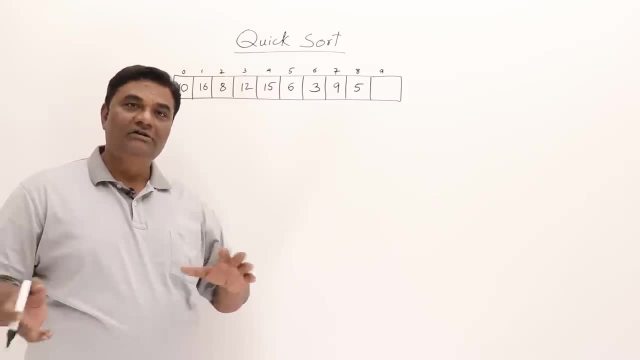 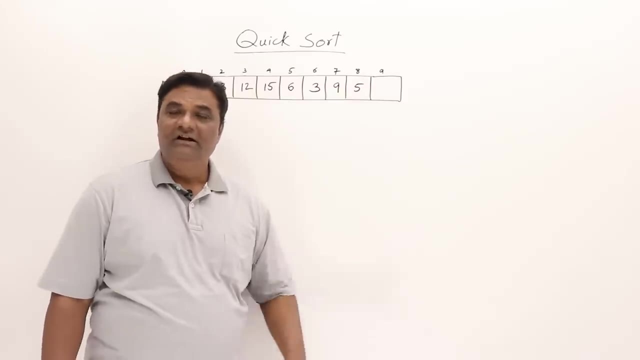 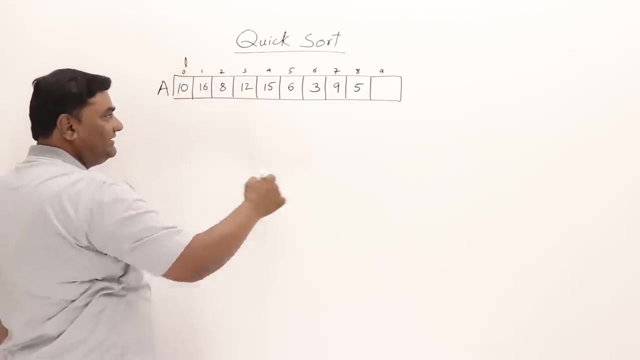 it will split the problem into sub problems and solve those sub problems. so let us see how it works. so I'll make initial setup first of all, then I'll show you the working. so the initial setup is: this is l- low- that is the beginning of a list. and this is high- that is end of a list. 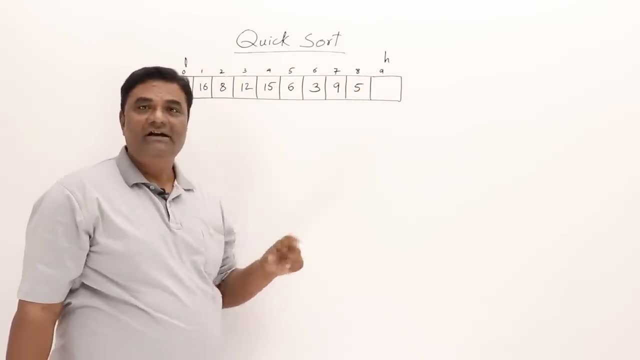 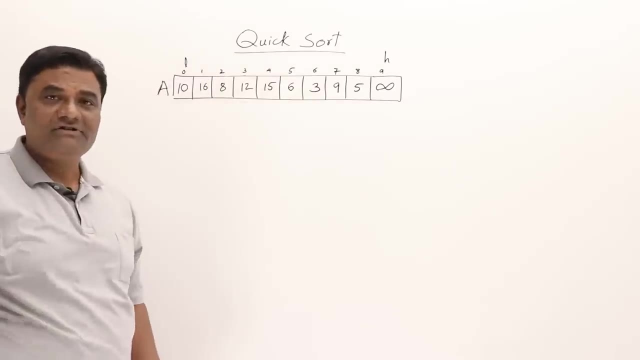 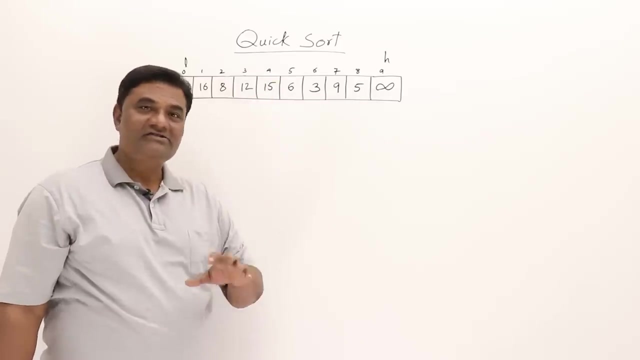 I have total nine elements. this place is empty. I have taken it. now I will add here infinity. that is maximum number. infinity is not defined in computer, so we take some maximum integer that will act as end of the list. list. like in strings we have slash, zero, null character. that is string terminator. here we 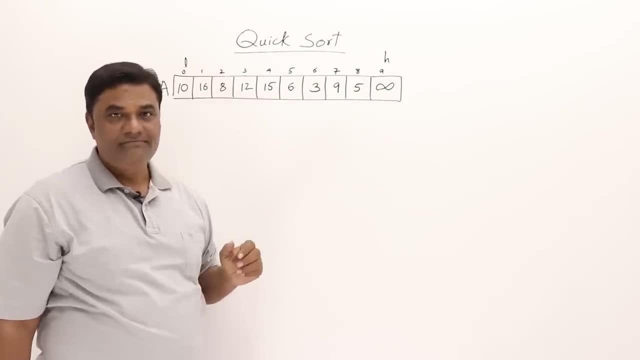 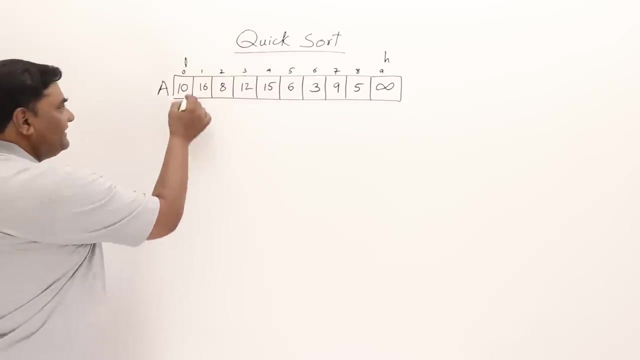 have taken infinity to show the end of a list. otherwise we should know that there are nine elements or 10 elements or 20 elements. we should work out according to length. instead of that, we prefer taking end of list marker, then first element i will select as pivot. 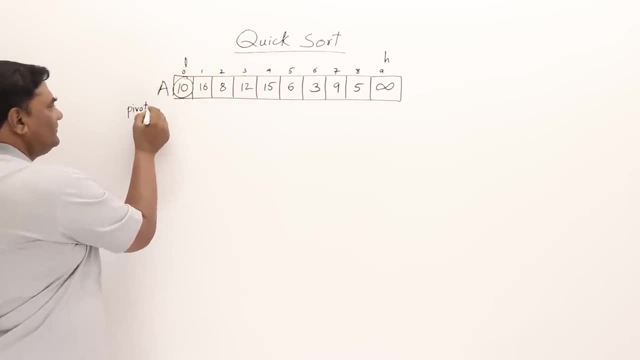 so pivot is 10, pivot is 10. so it means i want to find the sorted position of this 10, where this 10 should come. 10 should come at a place such that all the elements smaller than 10 should be on left side and all greater should be on the right hand side. for that i should check. 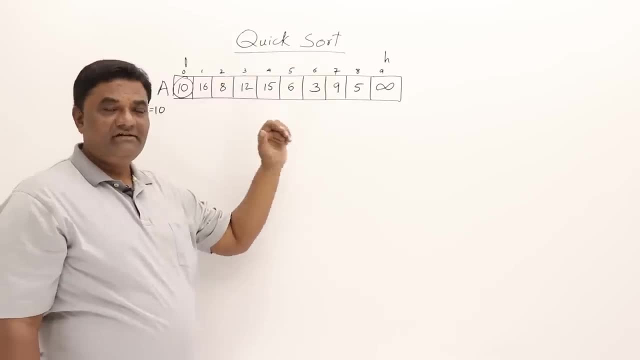 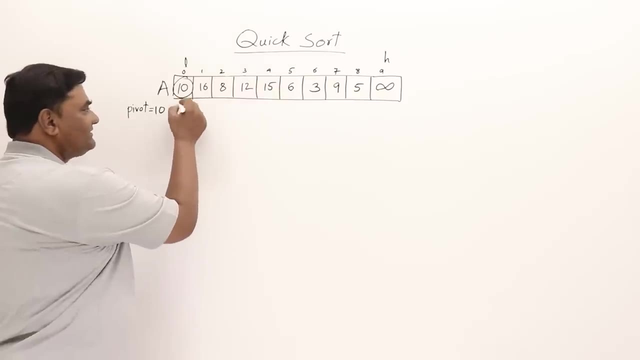 if any greater number this side, i will send it on that side. if any smaller on that side, i'll bring it this side. so for doing so, i will take i, starting from pivot, and j starting from infinity- i will search for the elements which are greater than 10, that's. 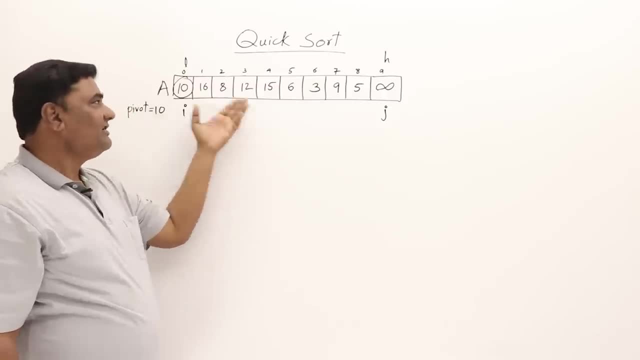 pivot and j will search for the element which are smaller than pivot so that they can exchange the numbers. all right, so i, at most it will be 10, and i will search for the elements which are greater than 10 and i will stop at infinity j, it will at most stop at pivot maximum if it is not getting. 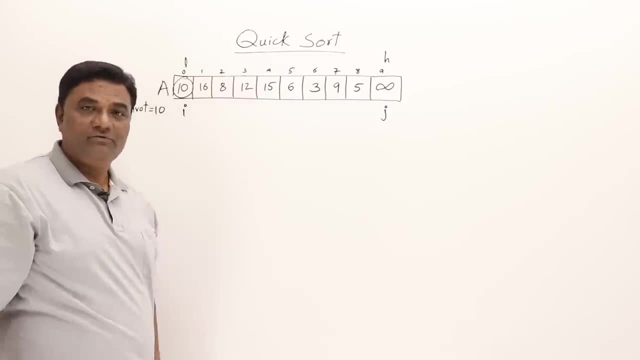 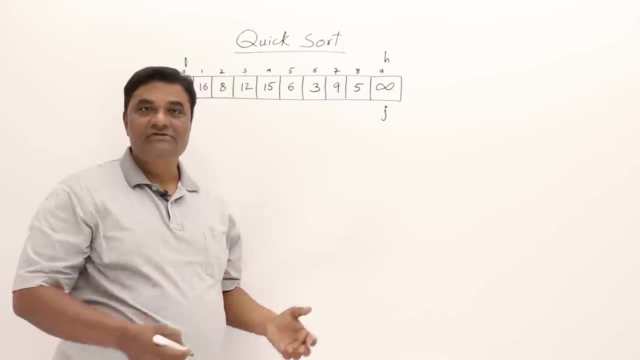 anything it will, at least, at most it will stop at pivot. now let us see the procedure. the procedure: what we will do now is called as partitioning procedure. first i will perform the procedure, then we'll write, then i will write down the algorithm for partitioning. let us start. 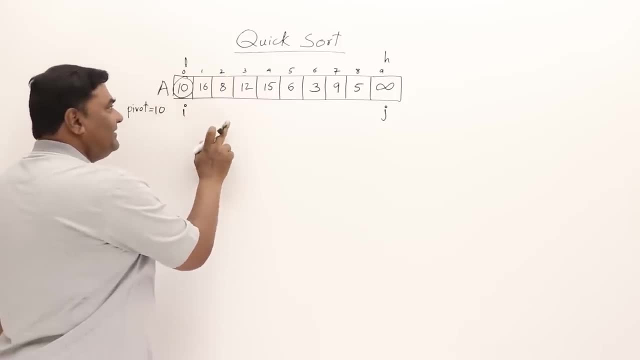 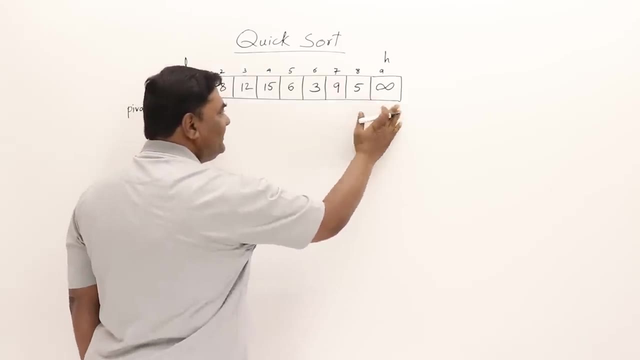 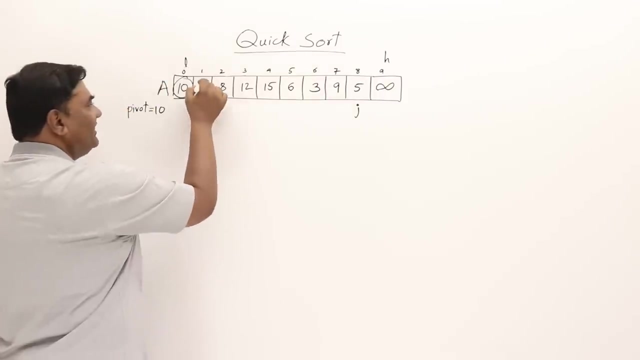 see. increment i until you find an element greater than 10. so the next element is greater than 10. only decrement j until you find the element smaller than or equal to pivot. that is 10. yes, this is smaller. exchange them: 5 comes here, 16 goes there. 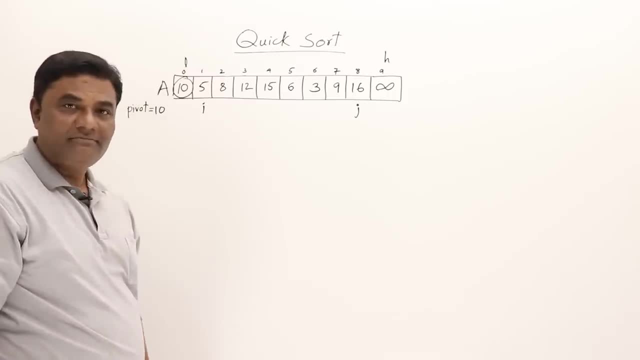 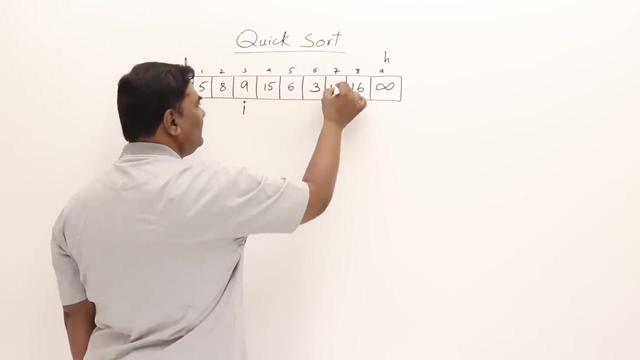 one swap. continue, increment i until you find a pivot. ie the pivot element is greater than pivot element 8. is it greater than pivot? no, 12 is it greater than pivot? yes, now decrement j until you get an element smaller than pivot. this is smaller. interchange them. 9 comes here, 12 goes there. 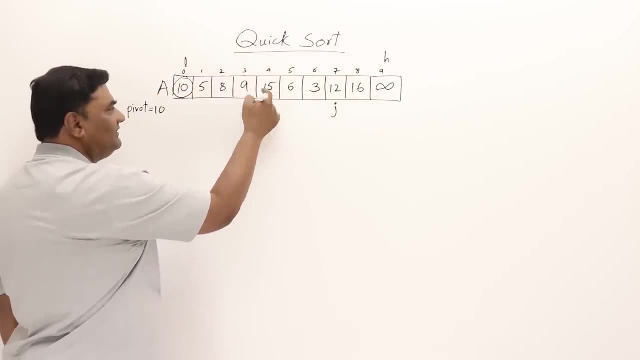 continue. i, this is greater. stop decrement j: this is small. stop 3, this side, 15, that side. continue. is it greater than 10? is it greater than 10? yes, I comes here. decrement J. is it smaller than 10? yes, this is smaller than 10. stop here, that's all. don't interchange I and J element, because I 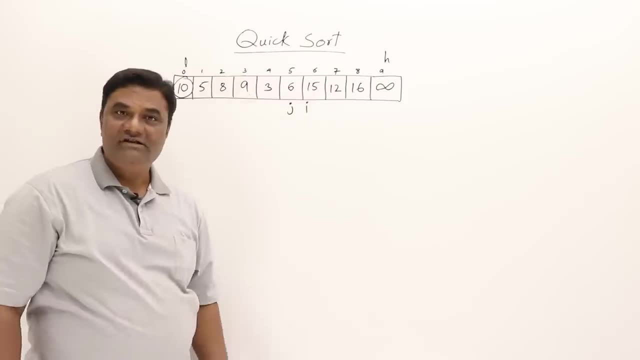 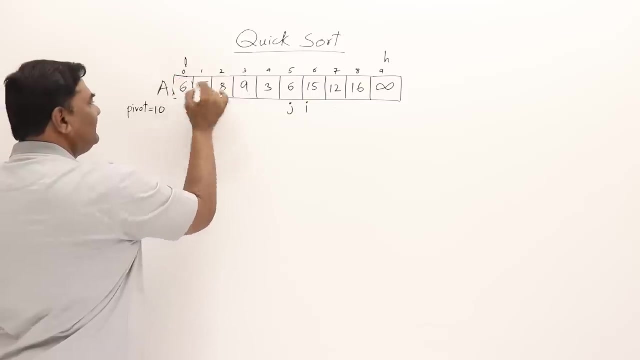 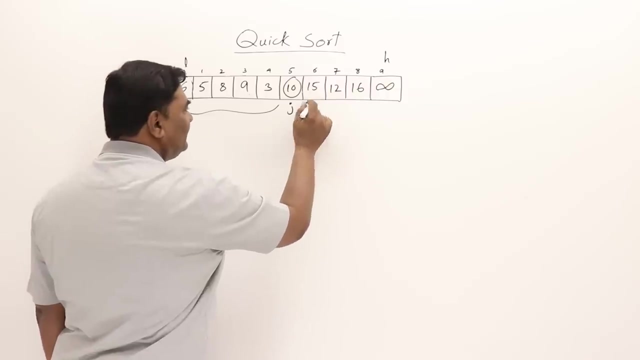 became greater than J. I has crossed J. it means we found the position of pivot. what is the position J? wherever J is pointing, that is the position of pivot. so send that element here and take 10 as this position. now this is sorted. this list is not yet sorted. and this list is not yet sorted. you can see that all the 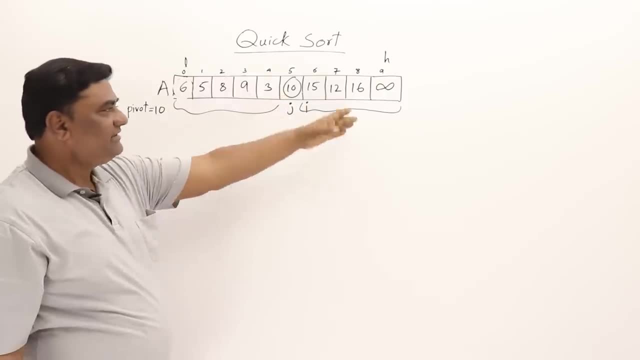 elements on this side are smaller than 10 and all the elements on that side are greater than 10, and these are not sorted. you can see that all the elements on this side are smaller than 10 and all the elements on that side are greater than 10, and these are not sorted. 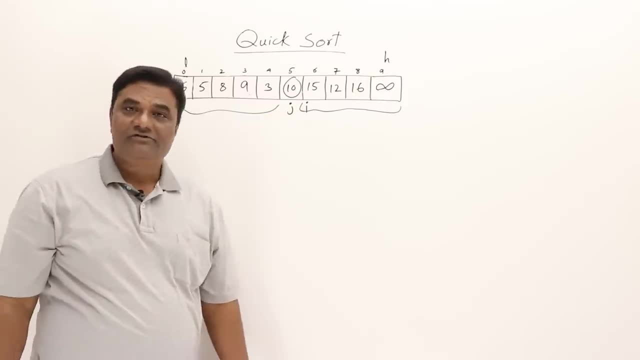 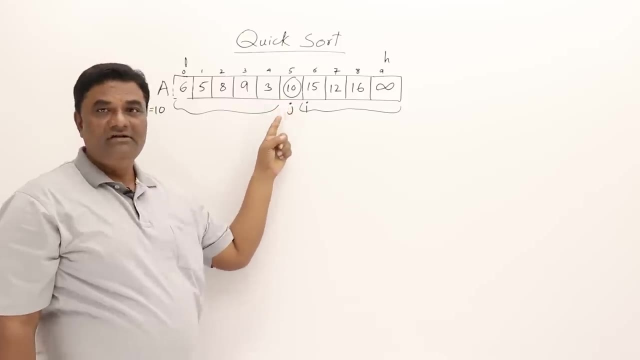 you can see that all the elements on this side are smaller than 10 and all the elements on that side are greater than 10, and these are not sorted. and even those are not sorted. we have to sort them then. who is sorted? 10 is sorted, pivot is sorted. this is the partitioning position. this is the 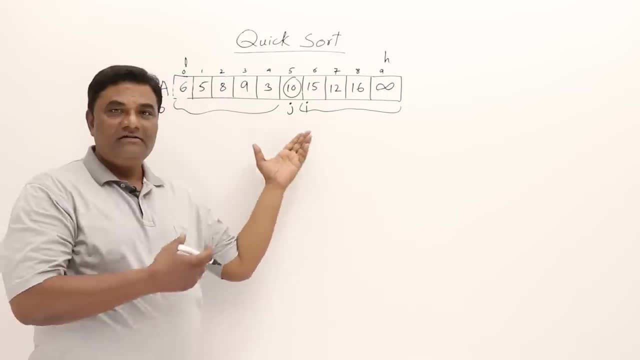 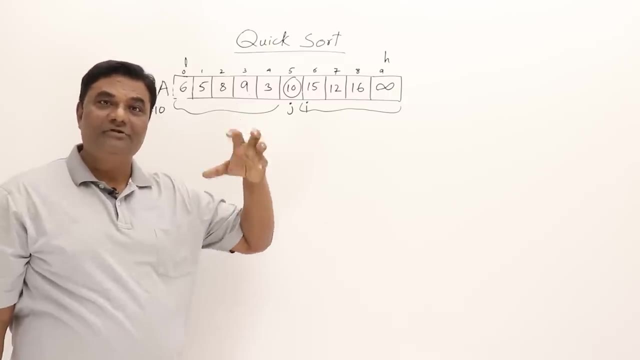 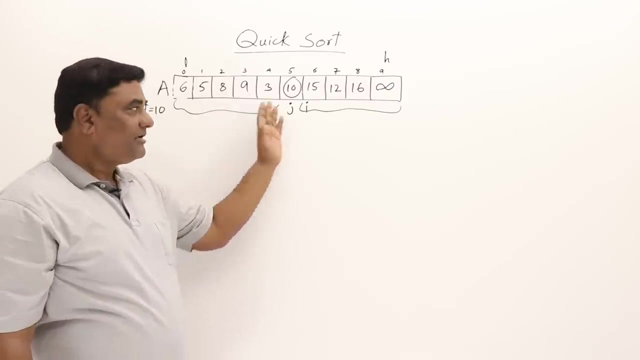 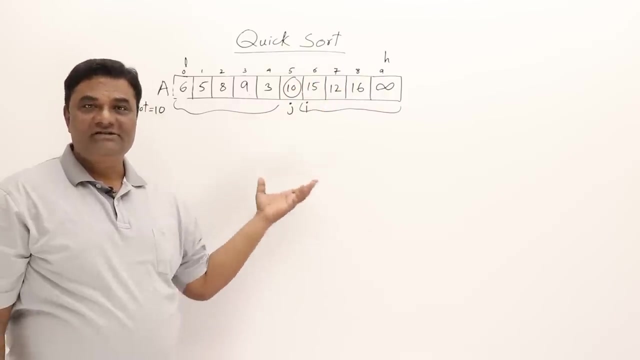 partitioning position. this is how partitioning position works. I have shown you the partitioning procedure, which has worked on one list and found out the position of a pivot element. now break this, perform quick sort recursively. perform quick sort recursively on either side. so that's it. this is the partitioning method. this is followed by. 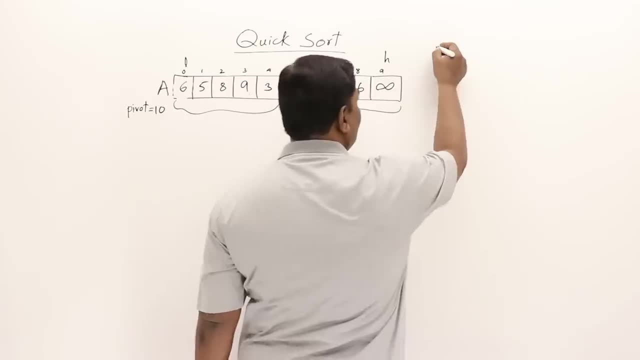 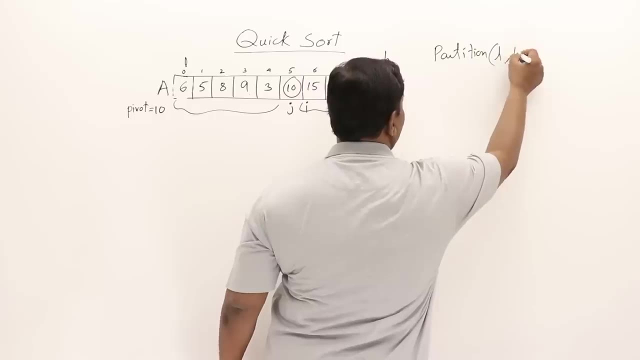 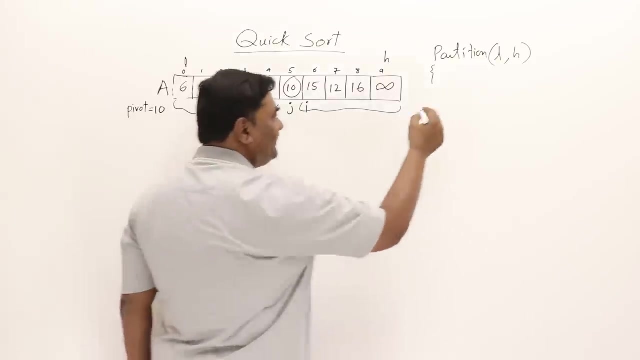 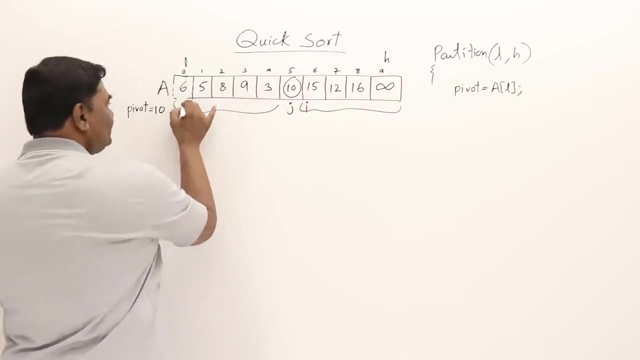 quick sort. let me write on the piece of code on this one partition. it takes low and high as a parameter. then what it does, select first element as pivot. so pivot is a of low. then I was starting from here, J was starting from here, so I will be at low. 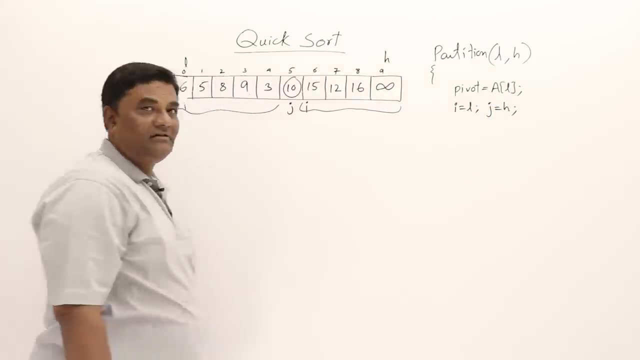 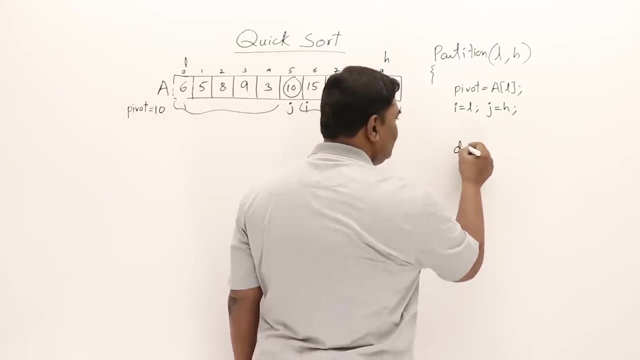 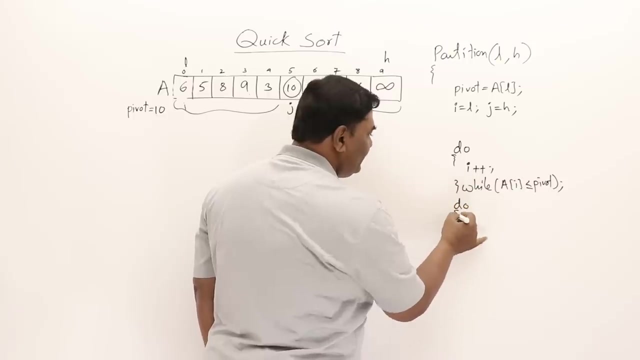 and J will be at high. then what we did with I? I was incrementing until it finds an element greater than pivot, so it was incrementing. if the element is a smaller than or equal to pivot, do I plus, plus, while a of is less than or equal to pivot, and similarly decrement J until you get an. 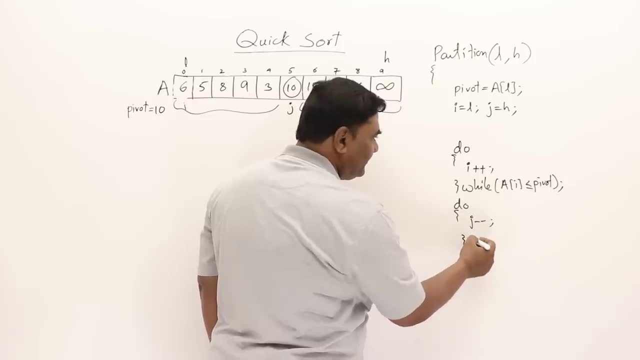 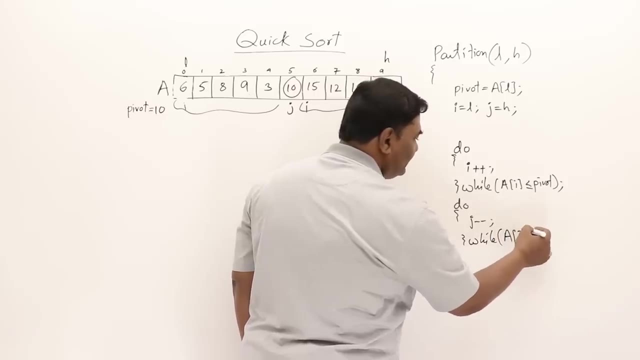 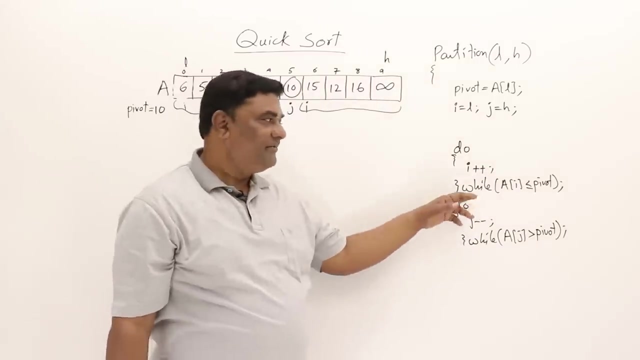 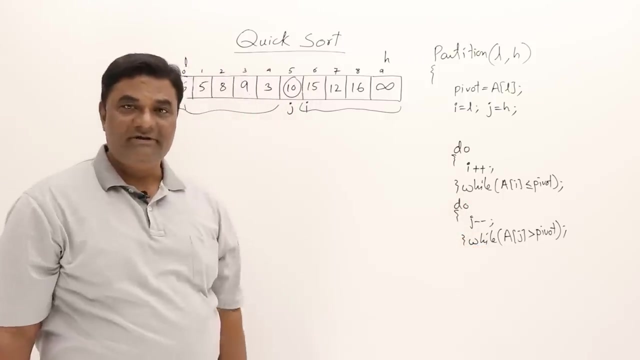 element smaller than or equal to pivot, while a of J is greater than pivot. so I will stop if it is getting any greater element and j will stop if it is getting any smaller element. So I have written the termination condition here. Then what to do? 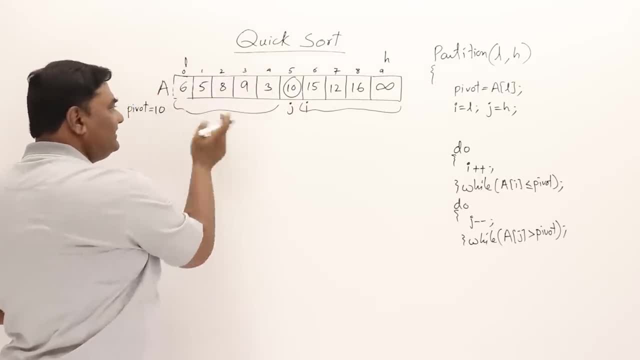 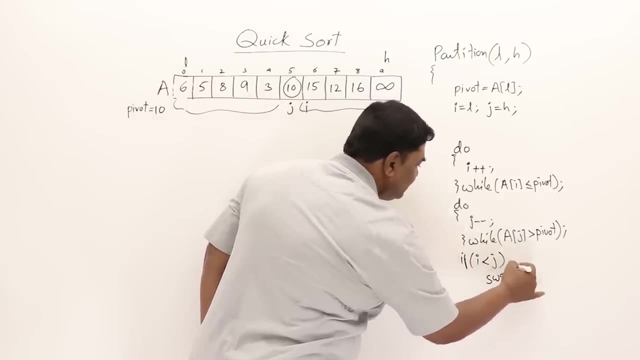 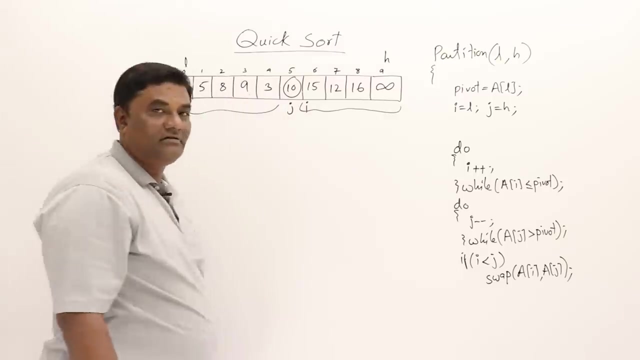 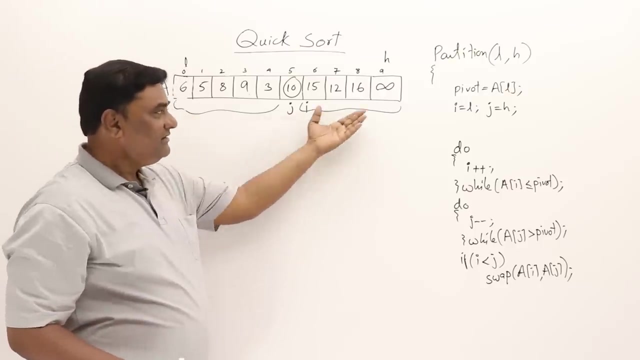 If i is on this side and j is on that side, only then interchange the elements. If i is less than j, swap a of i with a of j. This is just one comparison. Then again, continue i increment i and continue decrementing j and compare them and swap. 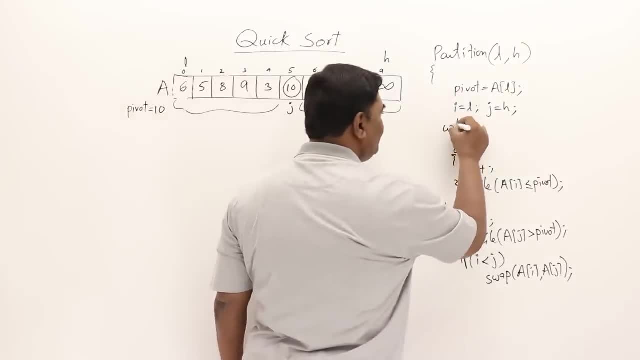 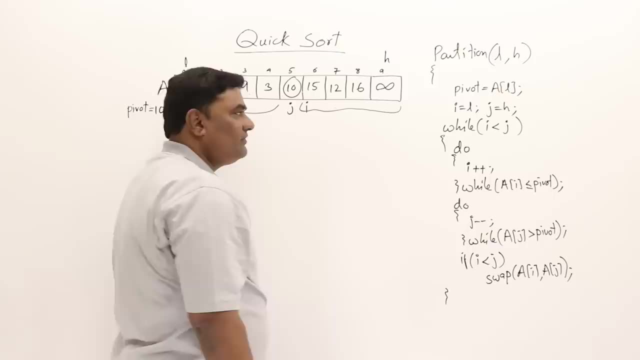 So this process has to be repeated, So I will write down this whole thing in a loop. How long I should do this while i is less than j? This I should continue as long as i is less than j. If i became greater than j, 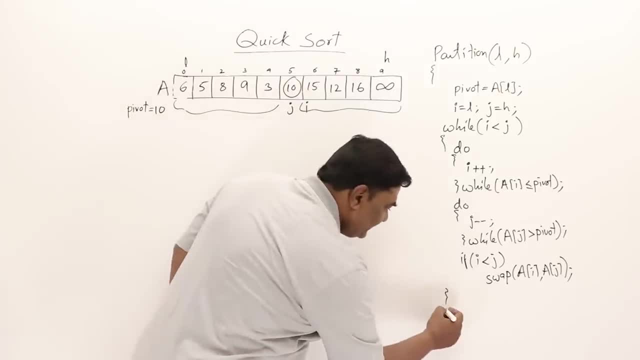 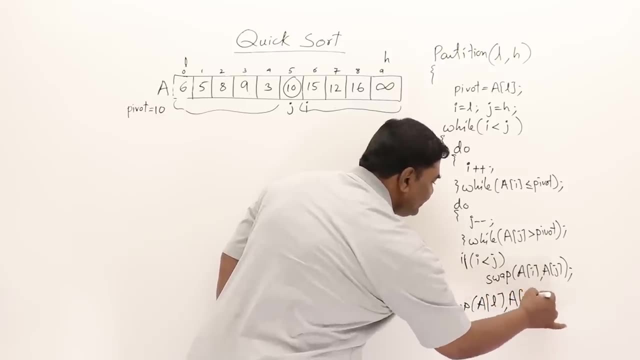 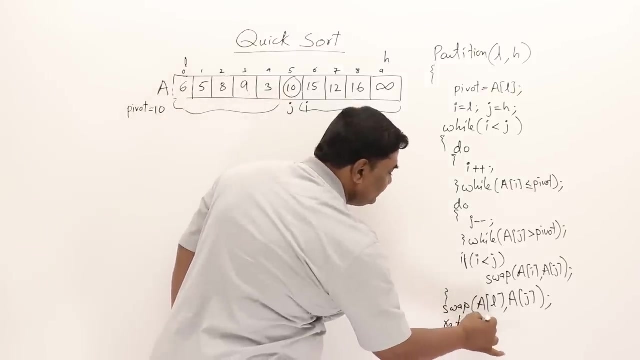 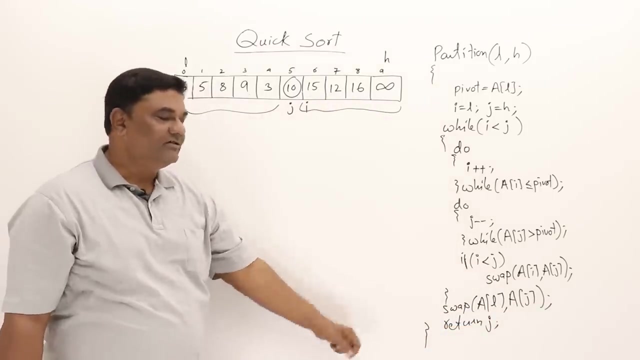 it will stop and here it should interchange, swap a of low with a of j. So swapping of pivot element should be done with j and return j. That is partitioning position. That's all. This is a partitioning algorithm. How quick sort works. 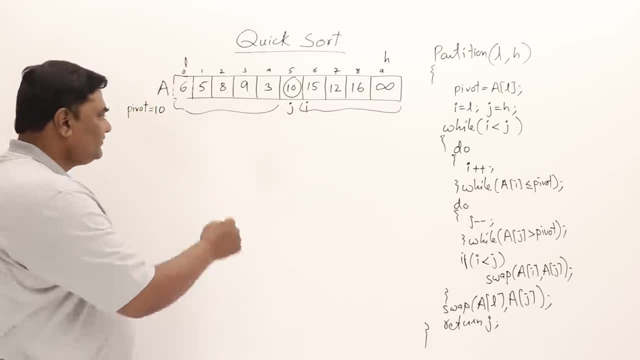 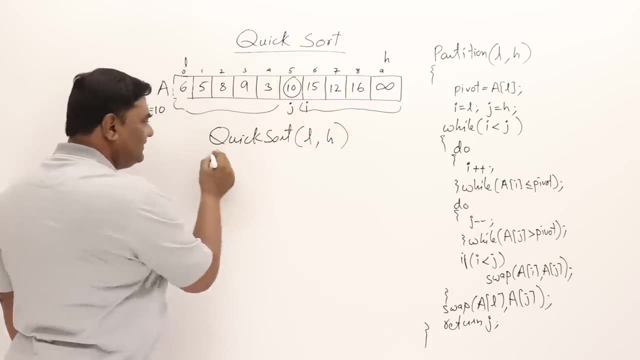 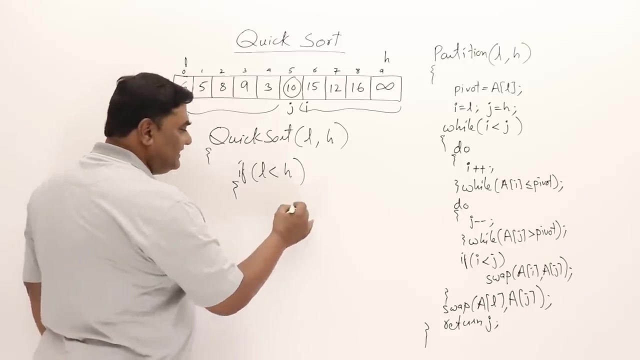 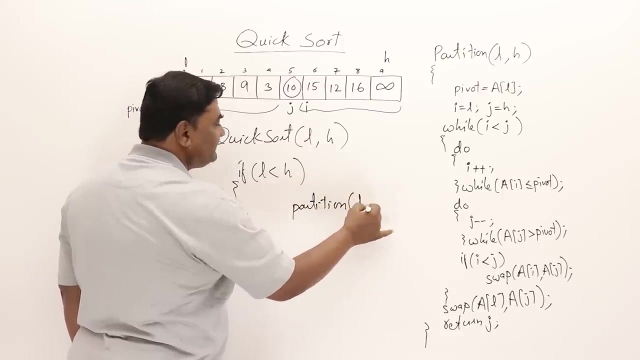 So this is just partitioning. Let us see how quick sort works. Quick sort, It will take low and high. If low is less than high, means at least there are two elements. If so, then it will call partition algorithm by passing low and high. 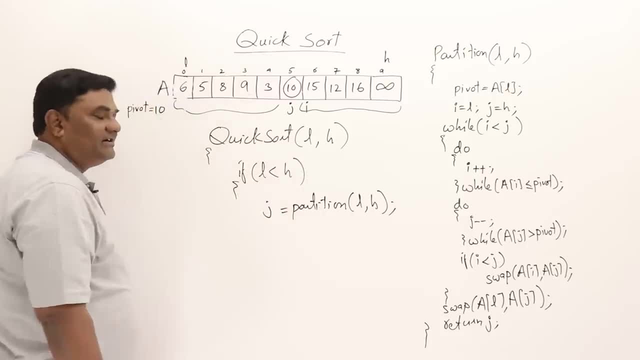 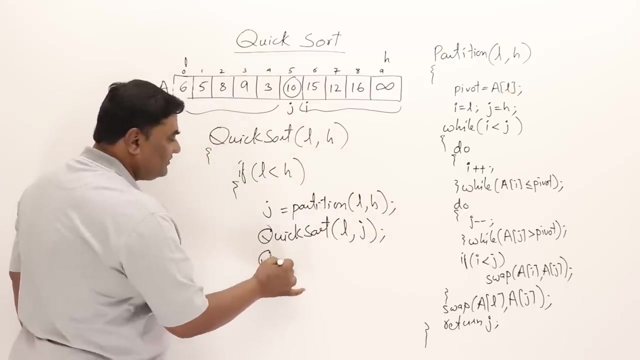 And that partitioning algorithm will return j, The position where the partitioning is done. Then it will perform quick sort on left hand side That is low to j, And it will perform quick sort on right hand side from j plus 1 to high. 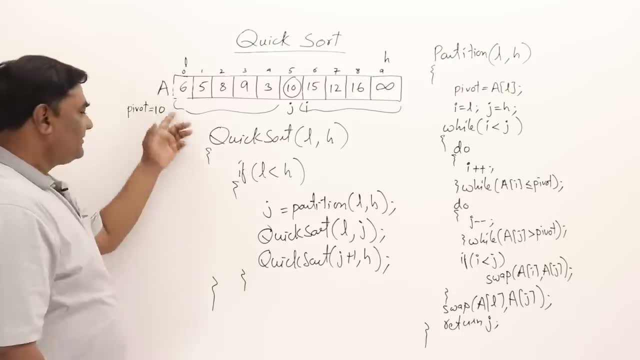 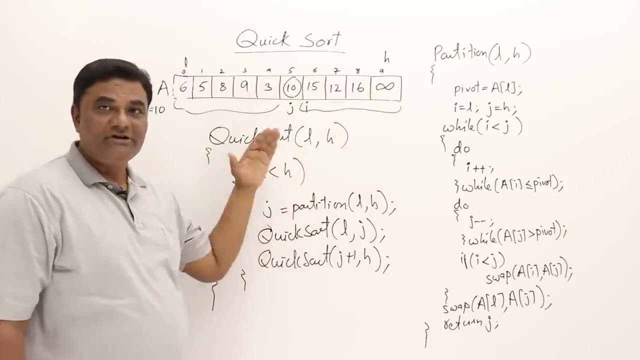 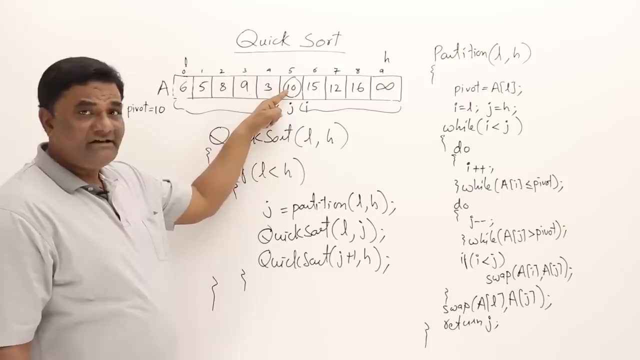 That's it. So it will perform this part. perform from low to j And this perform from j plus 1 from here to this one. Perform quick sort on 2.. Now, one thing I can show you here. This is already sorted. 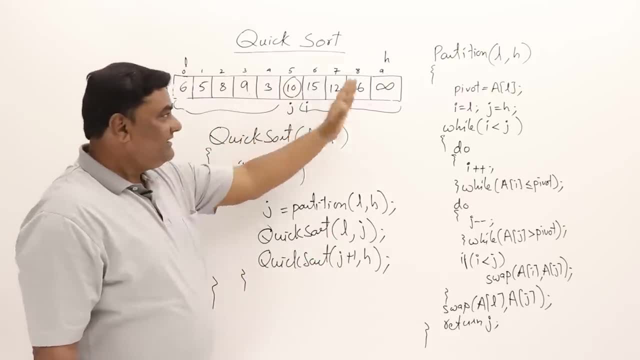 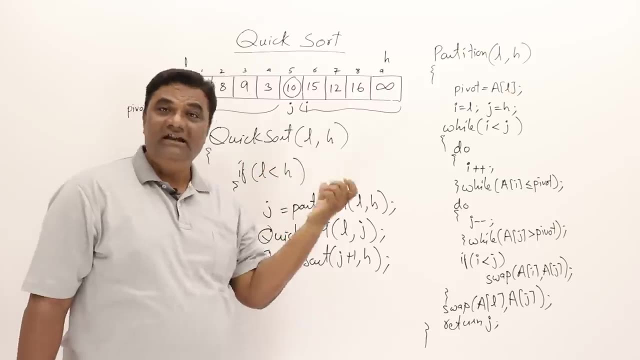 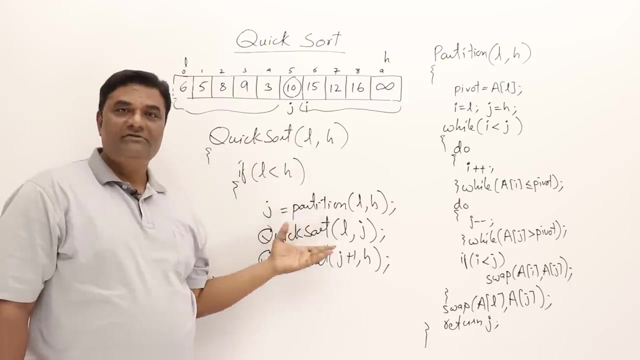 Why do you include? j See right hand side list is having infinity. Then where is the infinity for left hand side list? So this sorted element will help as an infinity act as an infinity for first list. So this is a small piece of recursive quick sort which is using this partitioning. 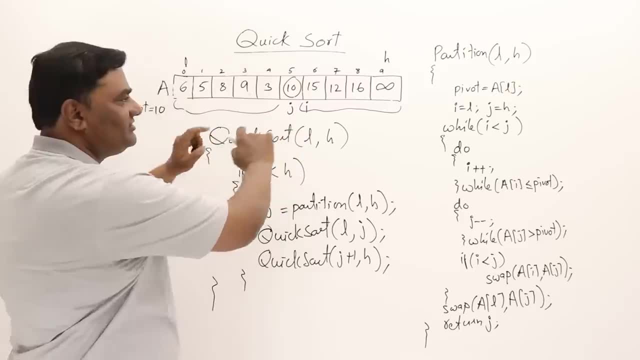 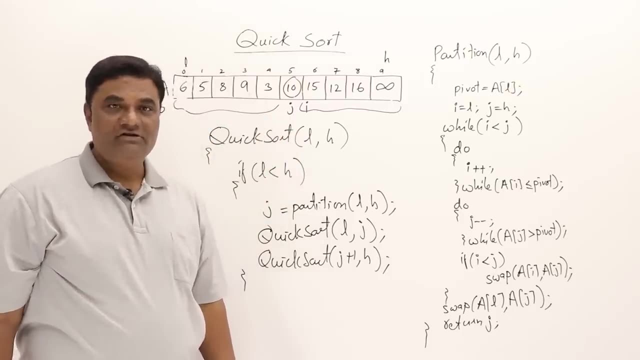 Partitioning was finding the position of pivoting. The position of pivot by taking i and j. That's all. Watch next video for analysis of quick sort.